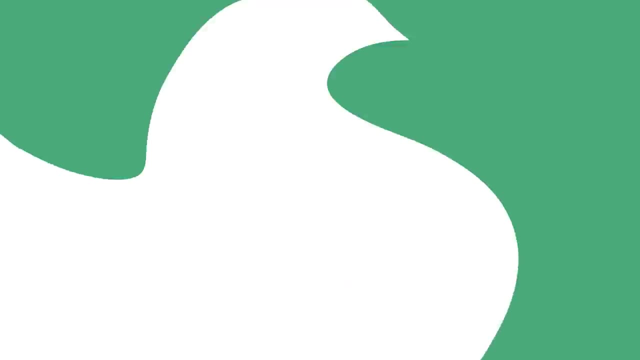 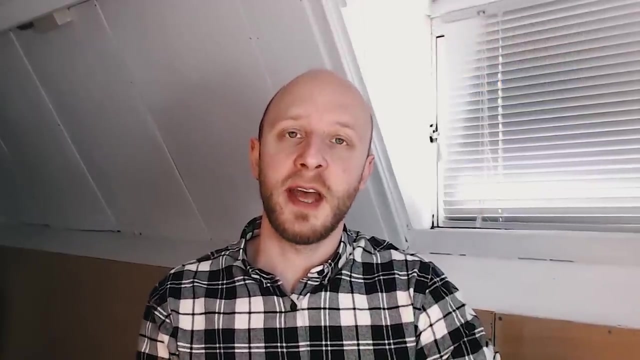 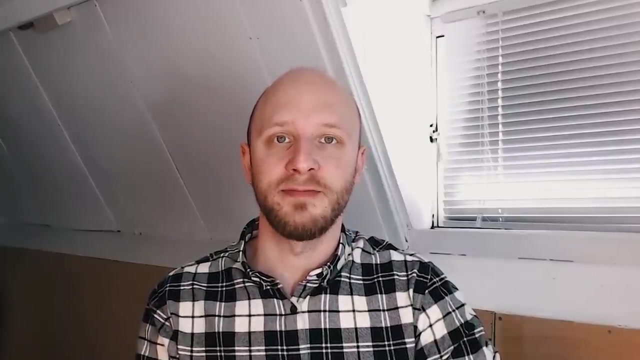 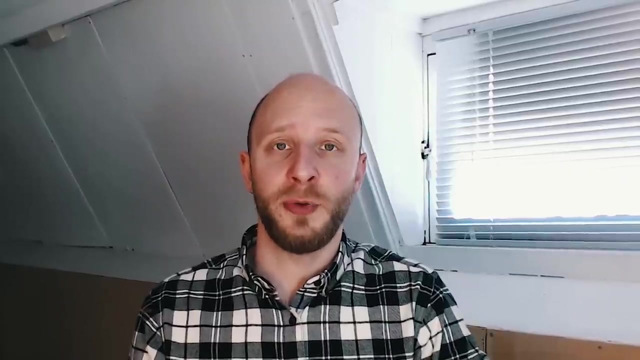 Hey there, You might have seen this video in which I explain how to draw like Kim Young-ji. Now, one of the main takeaways in that video is that Kim Young-ji is a master in using perspective, So let's take a deep dive in understanding how it works Now. Kim Young-ji is very hot right now. 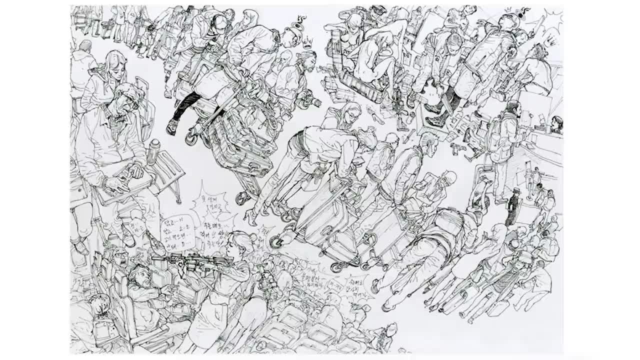 and if we look at the drawing like this, you can actually see that he's doing more than just making a drawing. He's actually telling a story And he's doing this by using several perspective grids in one drawing. He's actually using five different grids to tell a story from standing in line in 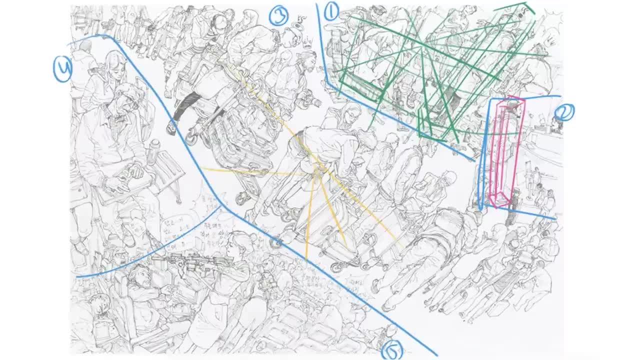 the airport to getting on onto the airplane, And in these grids he's just following the rules of the grid, right? He's just drawing boxes and filling them with different forms. Now I don't want to sound like this is easy, because he's filling them with pretty complicated forms like: 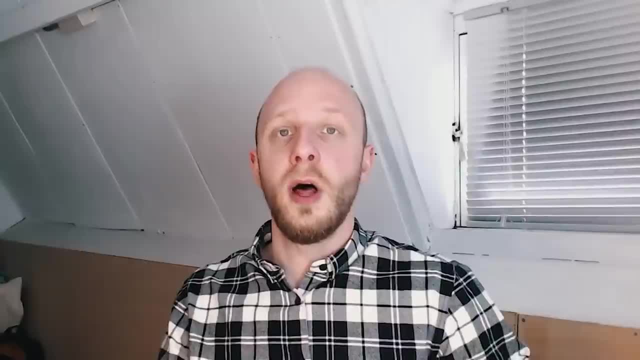 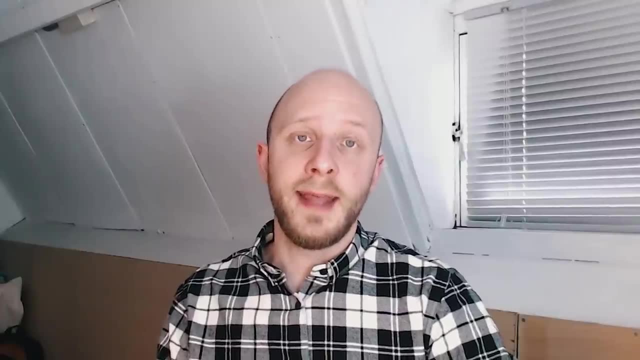 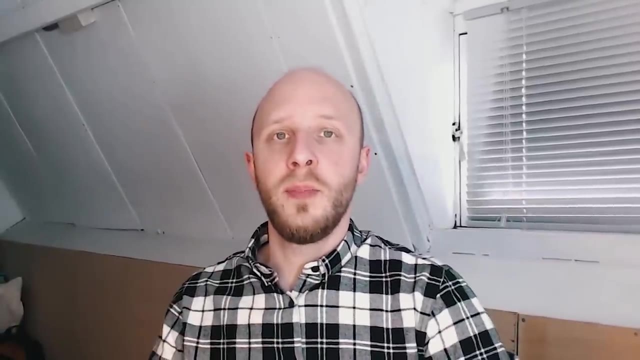 people, and in other drawings These are dragons or whatever. Although it's awesome what Kim Young-ji does, there's also a pitfall in being obsessed with his drawings, And that is copying his work instead of understanding the tools he's using. You know, it's fine if you copy his work, but this also means that you're actually. 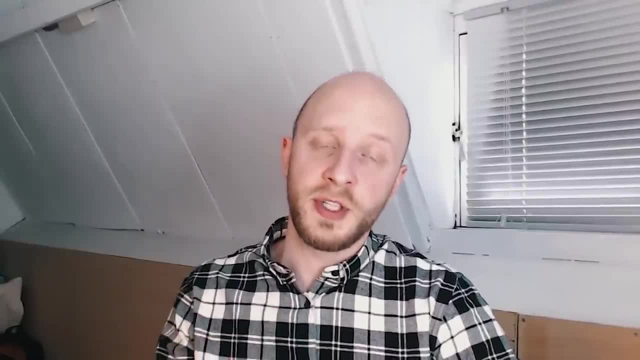 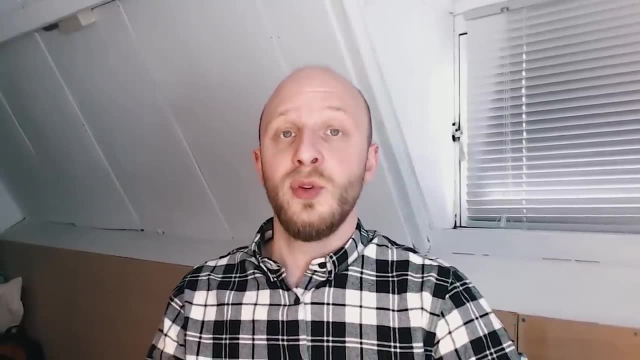 not visualizing your own imagination and sharing your vision with the world Now. to be able to share your vision with the world, you really need to practice the tools Now to do that. there are two things that are really important. The first one is that you need to practice the tools Now to do that. there are two things that are really important. 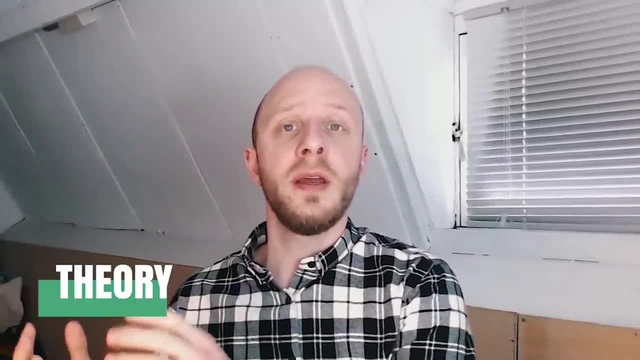 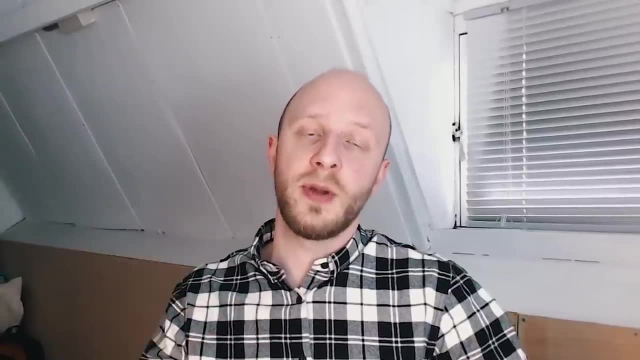 The first one is that you need to practice the tools Now. to do that, there are two things that are really important. The first thing is understanding the theory and the second thing is practicing it Now. to practice perspective, I've actually created a video, which you can find in the description, And this is a 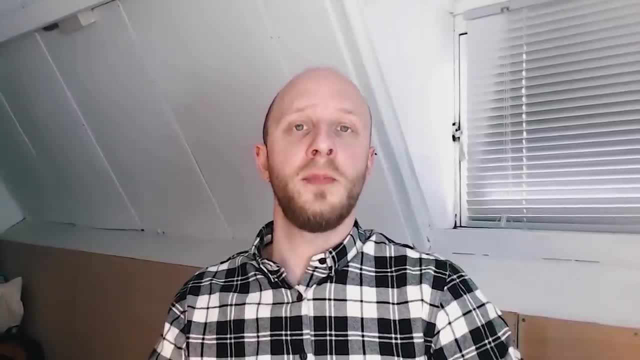 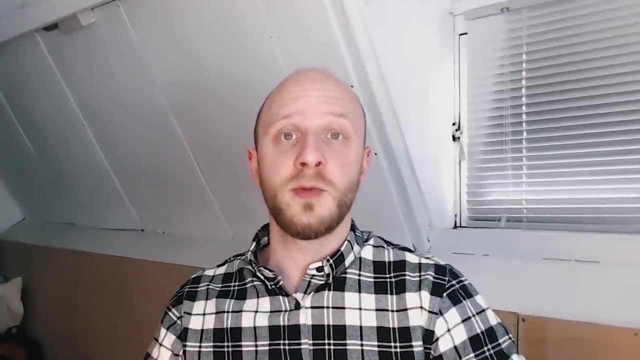 video with very specific workouts to slowly build up your perspective, knowledge and let it sink into your subconscious. But, of course, you also need to understand the theory, and that is what I'm going to be talking about in this video. We're going to be starting with very simple, one-point perspective. 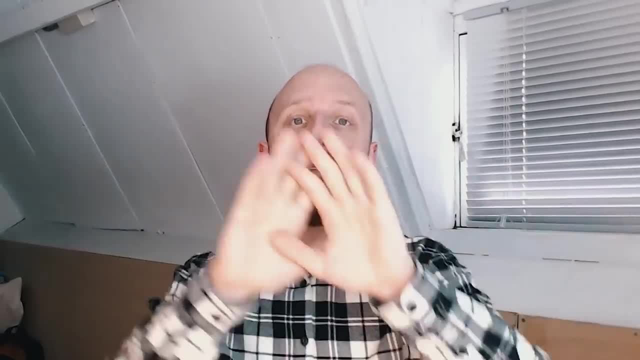 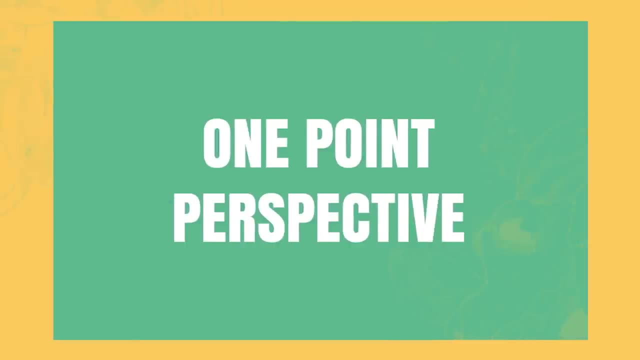 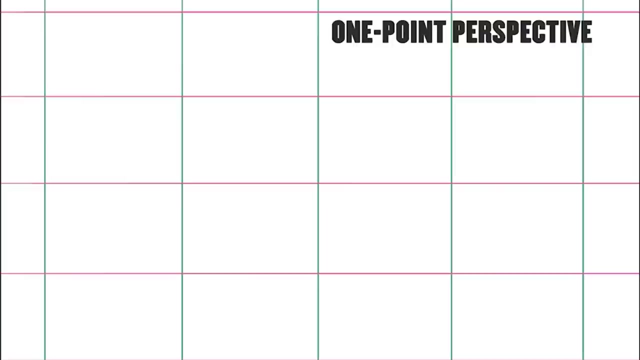 and eventually we're going to look at lenses and how they influence our perspective grid. So let's have a look. Alright, so let's start with the easiest perspective, a one-point perspective. Now, before I start drawing, you can already see that there's a grid in here with green. 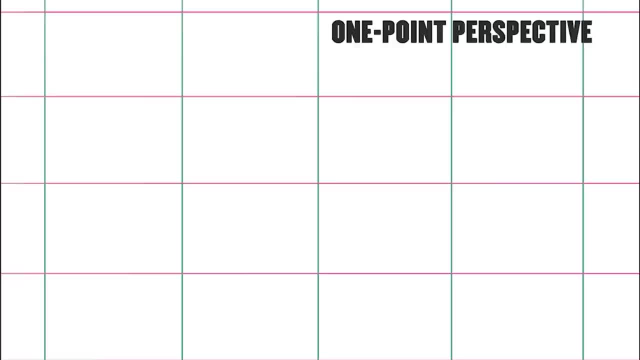 and pink lines. The greens represent the vertical lines and the pink represent the horizontal lines. This grid already gives us a guideline on how to draw in a one-point perspective Drawing. Now let me show you what I mean with this. We start with drawing in a horizon line over. 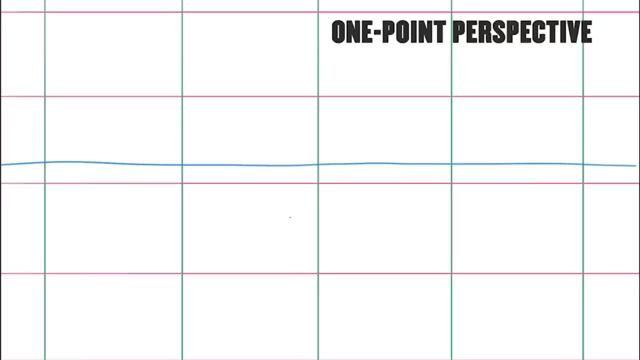 here and let's say, this horizon line has a vanishing point over here. I put a one in here because this is our first vanishing point. To create depth, we'll need to follow the guidelines from these vanishing points, which are actually radiating lines coming from this vanishing point. 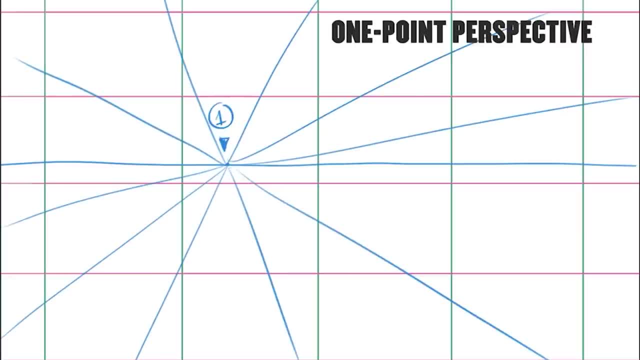 Like this. Now, if we want to draw a bar- let's say we have a box that goes towards this vanishing point- Then the front of the box is actually following the green and pink lines. So let's say we have a box over here. 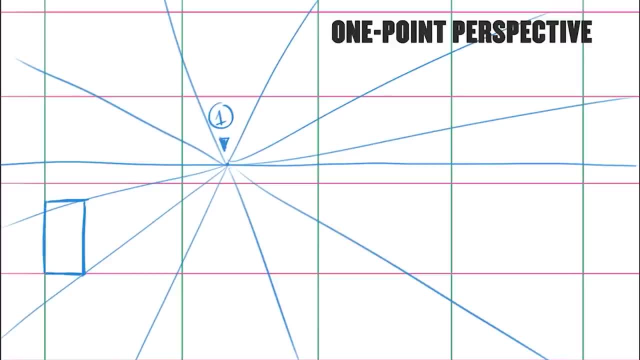 Then you'll see that these vertical lines and these horizontal lines are just following the green and pink lines. But when we go towards the vanishing point then we need to follow the blue lines. So we go towards here and then we go up again. 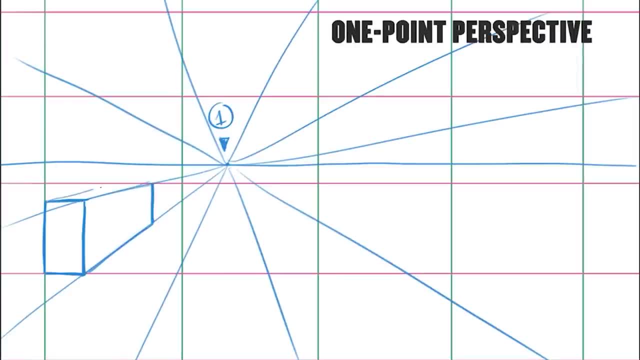 Then already here, So we can see that the green line is the corner of the box, And this one also goes towards the vanishing point, So we can just see the top of the box. So this is actually how we draw boxes in a perspective grid. Now let's say we want to. 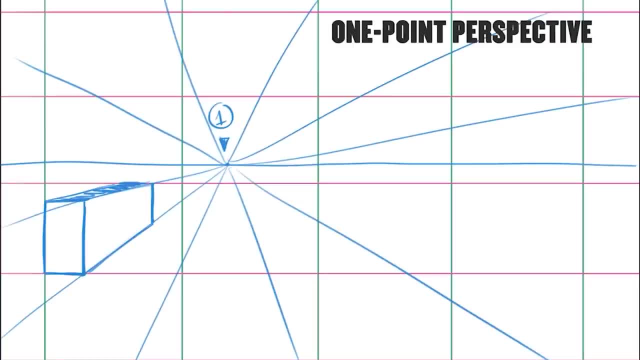 draw something more complicated. Let's say we want to draw a street that goes towards the horizon. We're going for a road trip. Next to these streets are standing street lights And let's say we have a very distant street light standing over here. This is a really small street. 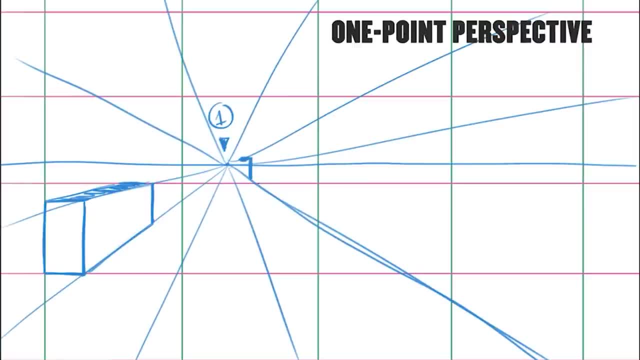 and it's really far away Now to measure our next street light. we know that the front of the street light actually touches this line. So let's say, we draw this street light over here. Now the back of the street light also has a line And here we're drawing it. but you'll 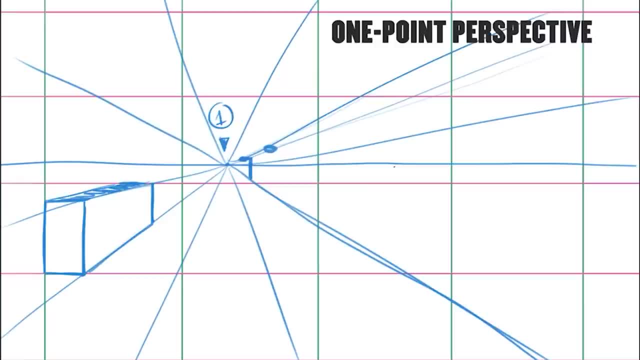 need to try to understand, to visualize this instead of literally drawing it. We've drawn in this line and now we're actually again following the pink lines, Where we here we're touching the back of the street light, And then we go down and we follow the green lines, So now we actually have another street light. 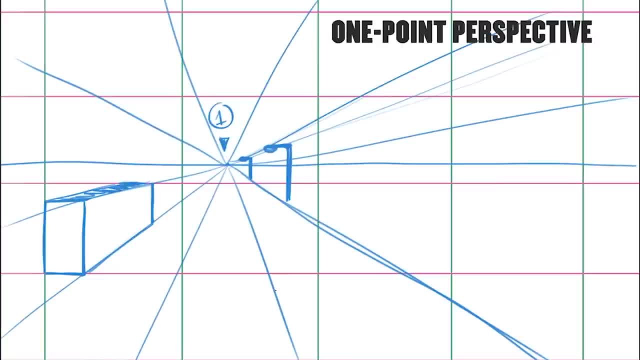 Now, if we want to draw our third street light, it's pretty hard to understand where should we draw this street light? Is it over here, or maybe over here, or you know? if these are consistently far apart from each other, then we need to measure how far or where do we place our third street? 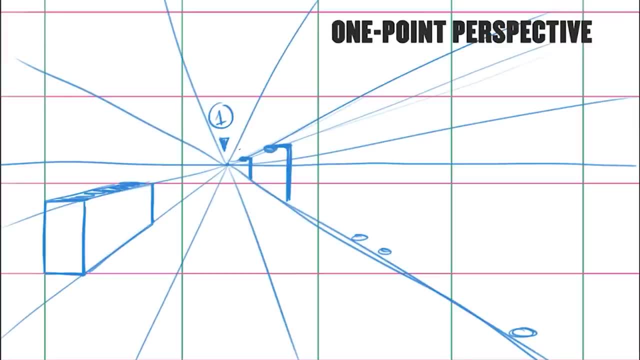 light. Now, there's actually a trick for this, because if we have these points, then this, this distance is actually one third of the distance that the next street light is. Now, it sounds a little bit complicated, but let's say that we do this times three, So we, this is our also another. 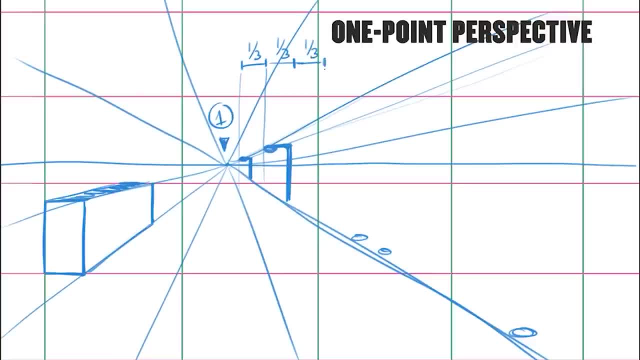 third, and this is our another third, Then this: so we started measuring from this line. then this is where we place our third street light, And again here on the top, we're following the pink lines and here we go down and we have, and we're following the green lines, And now we have three street lights. 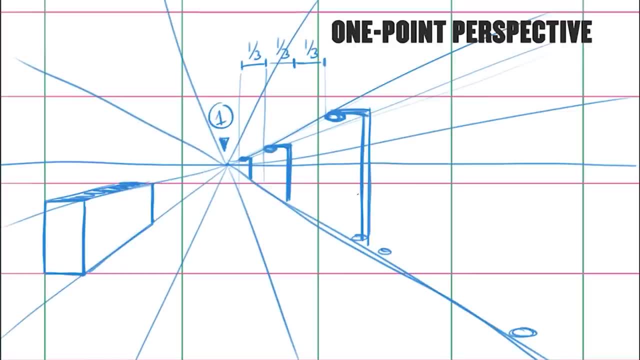 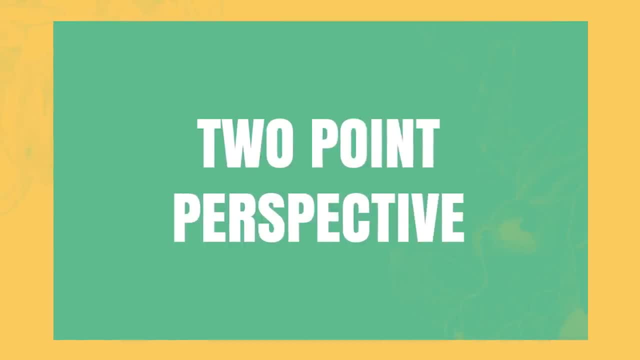 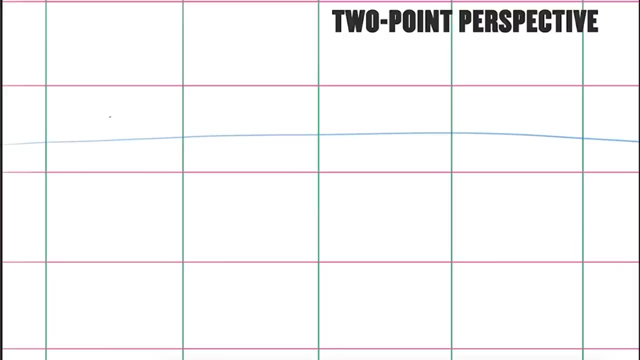 that are all the same distance apart from each other, and they're all similar. And that's how we start drawing in a one point perspective. Now, when we look at two point perspective, actually the same is going on as in one point perspective. So let's draw our horizon line, but instead of having one point, we have 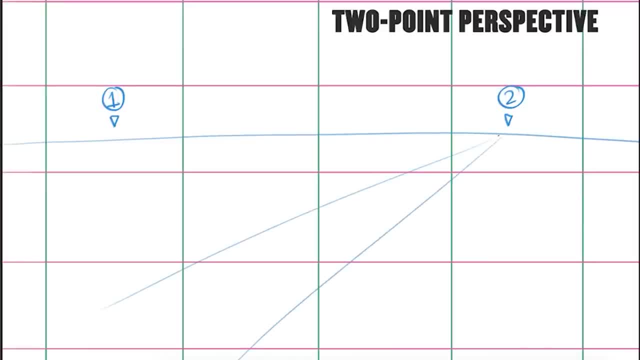 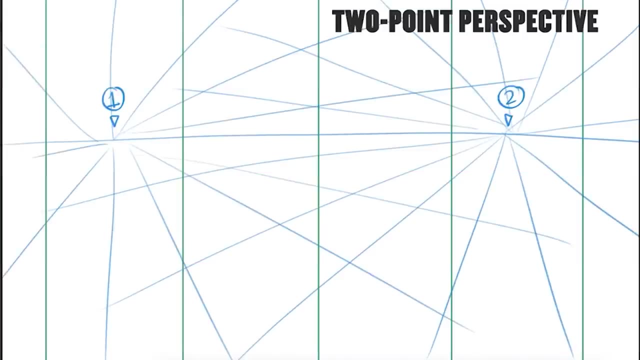 two points, with both the radiating lines that create depth. Now this actually has an effect on our current grid that we have with the green and pink lines, because the pink lines, which represent the horizontal lines, they don't exist anymore. We can just take them out because now we have an extra vanishing point that represents the 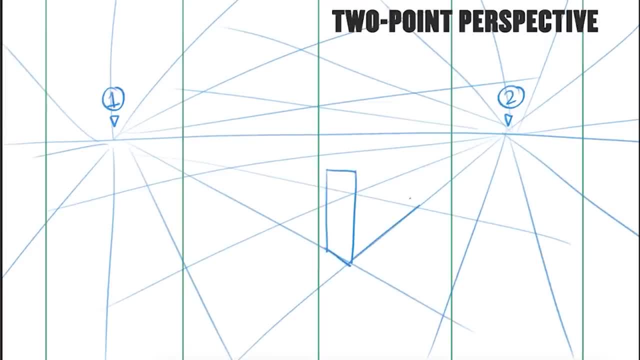 horizontal lines. Now this has an effect when we draw boxes, because now our horizontal lines actually need to converge towards vanishing point. In this case, the second or the first one doesn't really matter. Now, again, if we start drawing in street lights, you'll see that the top of these 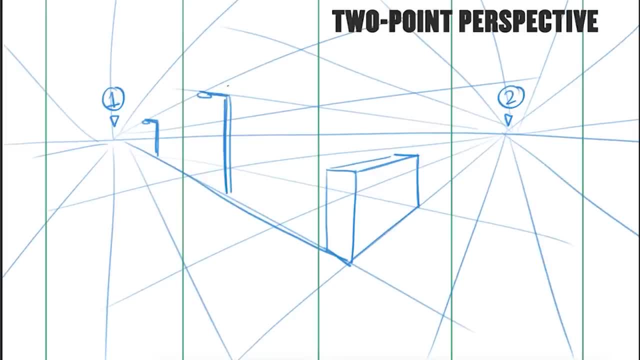 street lines, which are horizontal in the first image, are actually getting a bit of an angle here. You can actually see that on the third one, where the angle is really converging towards the second vanishing point. So here on the right we see a box coming to life. that looks kind of funny. 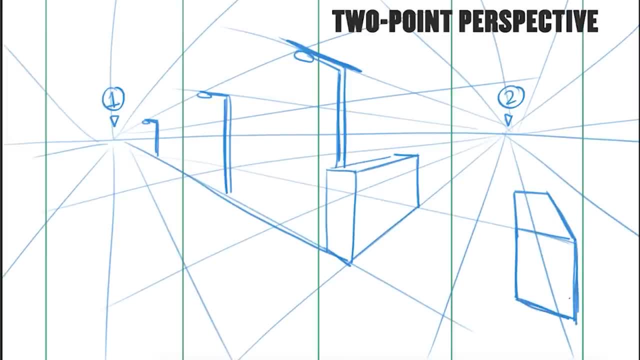 And the reason is because we can only see two sides of this box, Compared to the box in the middle, which has three sides. this really clearly communicates a box, while the box on the right communicates more like something else. Now, what's happening here is that distortion comes into play. 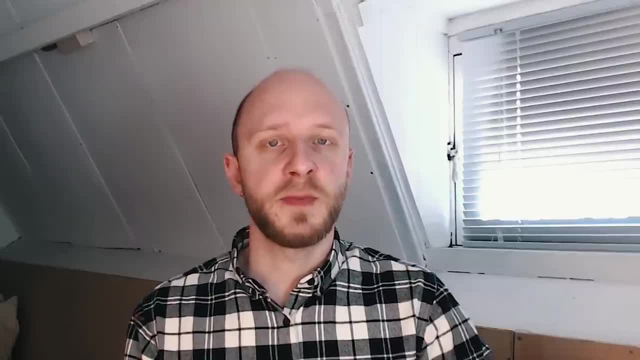 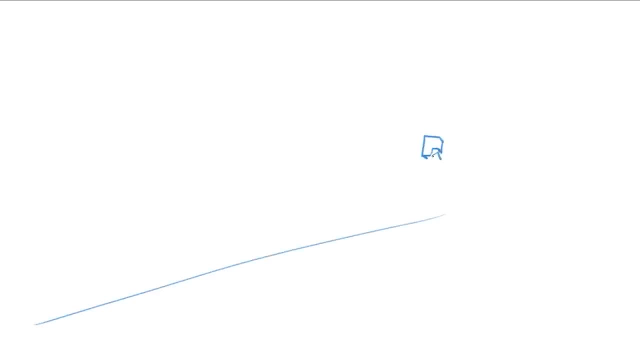 and distortion is something that explains when perspective is getting a little wonky. Now let me show you what I mean with this. All right, so let's say you're drawing on a wall, right, We have the edge of the ground here, and you're here standing and thinking and 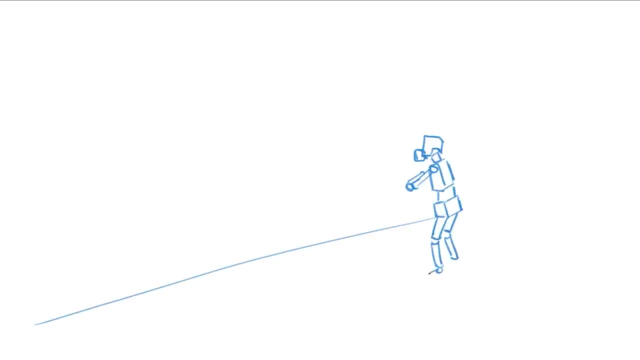 contemplating on what you want to draw. Now, if we hang up a piece of paper on the wall here, you can decide where you want to place your vanishing points. Now, the way I do this is by writing down VP on a post-it and literally placing it somewhere on the wall. 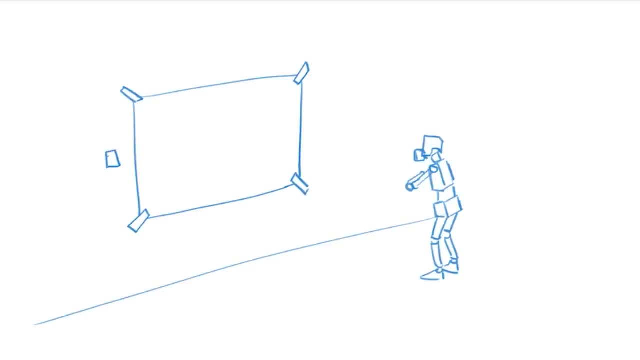 So let's say, we have a vanishing point over here which has VP, and we have a vanishing point over here which is VP. Now again we of course we have our horizon line which goes like this, with its radiating lines coming from the vanishing points, just like we had before. 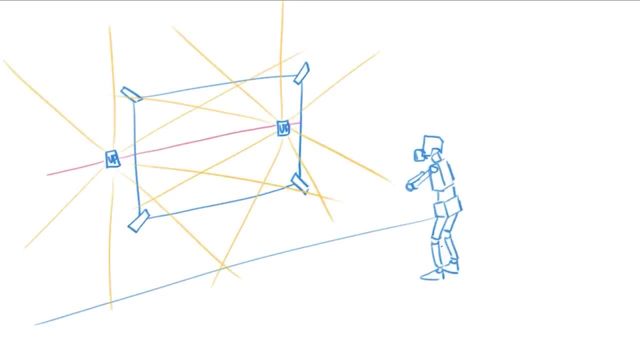 Now we can decide, as an artist, where to place these vanishing points. right, We could also say: we place one over here, all the way towards the left. It doesn't really matter where we place them, but it does have an effect on our boxes. So, for example, if we draw a box over here, 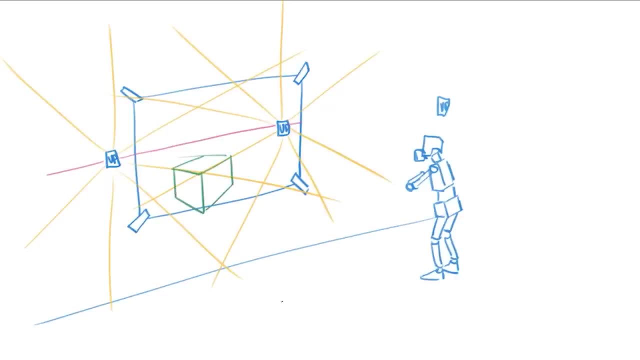 this box is just following the rules of the perspective grid and it looks correct. But if we start drawing a box over here, for example, and we follow the same grid, then this box is getting really strange. It's starting to look like this Now. the reason this happens is because when we start placing boxes on the outskirts, 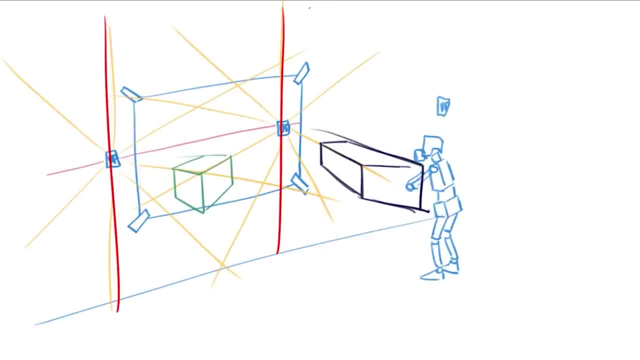 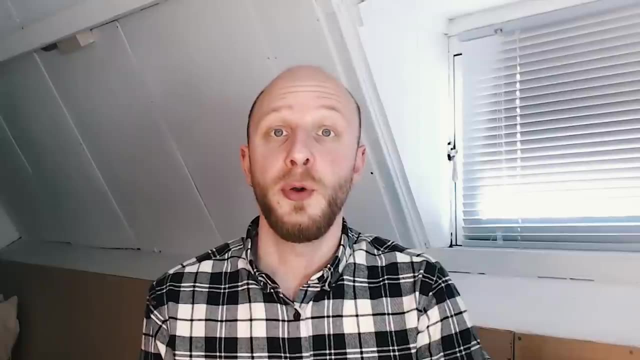 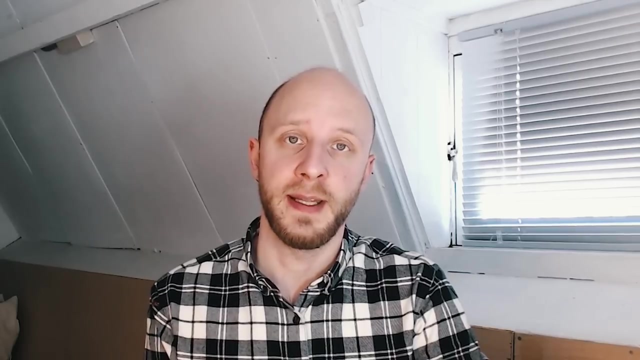 of our vanishing points, so that means in this area, then they become distorted. Although you can use distortion as a tool, I highly suggest you stay away from it because it interferes with our communication of realism. So choose vanishing points as far away from the page as possible. 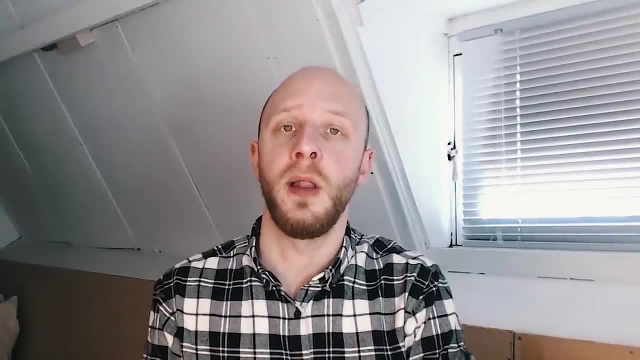 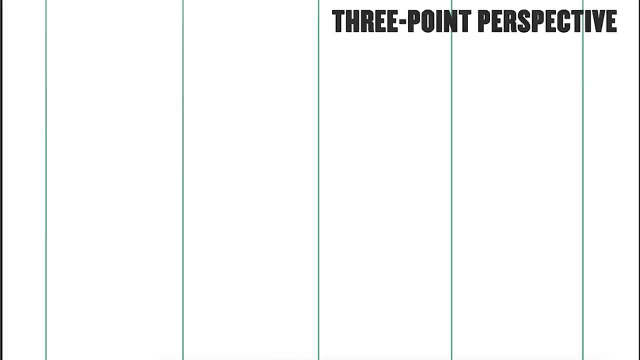 This makes your drawing easier and communicates form a lot better. All right, so let's have a look at a three-point perspective. You would have guessed it: a three-point perspective just has an extra vanishing point. If we draw another horizon line and add our existing vanishing points from the last one, we get actually the same image. 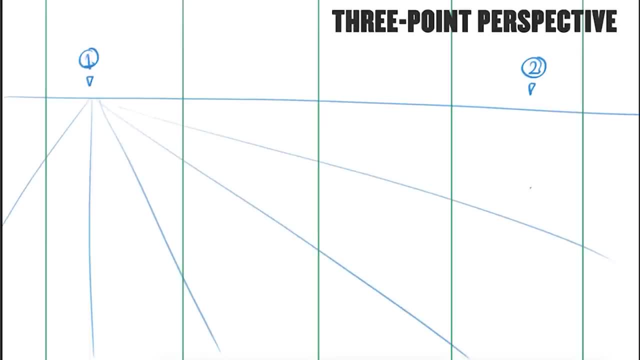 Now the extra vanishing point, or the third one: either goes above or below the horizon line, So in this case, let's choose a vanishing point that goes below the horizon line. Now also, this vanishing point has radiating lines, which has an effect on our last green grid lines. We can 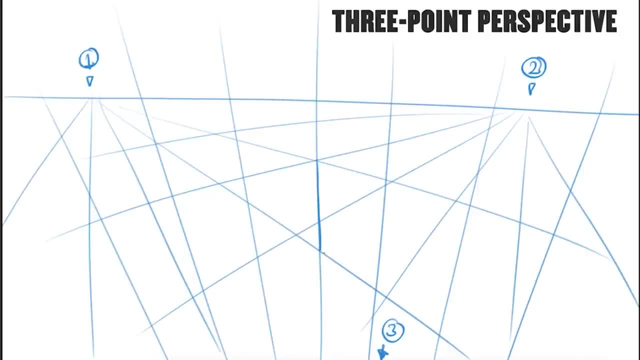 actually take them out. So let's have another look at our vanishing point. If we look out the entire horizon line, we'll see that the vanishing points are everywhere. Now this makes drawing a box, of course, a little bit harder, because all the lines that we are 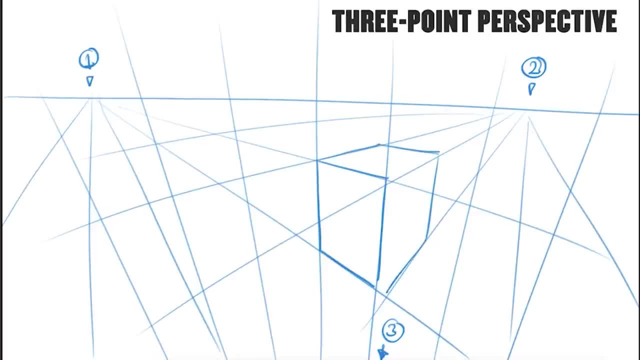 drawing are converging from some vanishing point, Either the left, the first one, the second one or the third one. Now let's see what the effect is on our street lights. So if we draw these street lights, you'll see that the left street lights are really kind of leaning towards the left. 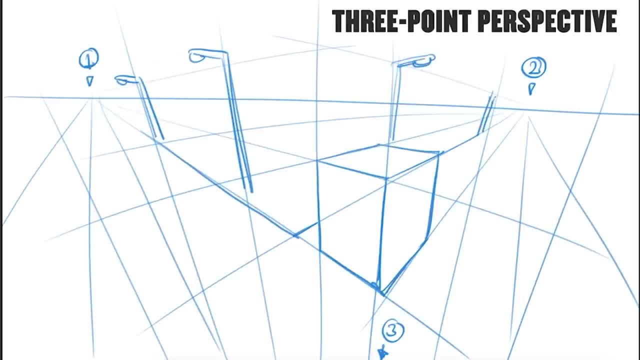 which seems to be unreal, But in this case they are really following the rules that we set up for this perspective grid, And in that case it's correct. So you can actually see that you, as an artist, can create whatever grid you want. It doesn't really matter, but you 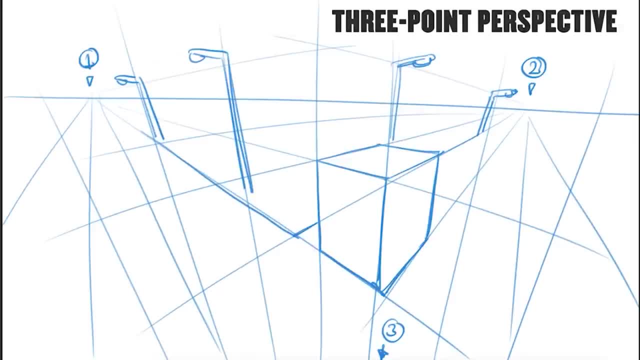 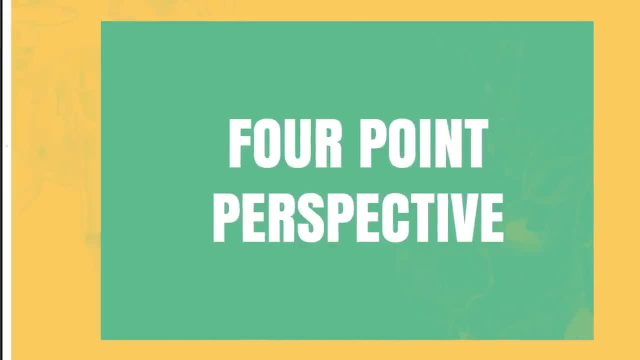 just need to keep following the rules you set up in your own grid or in your drawing. All right, For this video, I'm going to show you how to draw a street light, So let's get started. Four point perspective. Now, four point perspective, as you would have guessed. 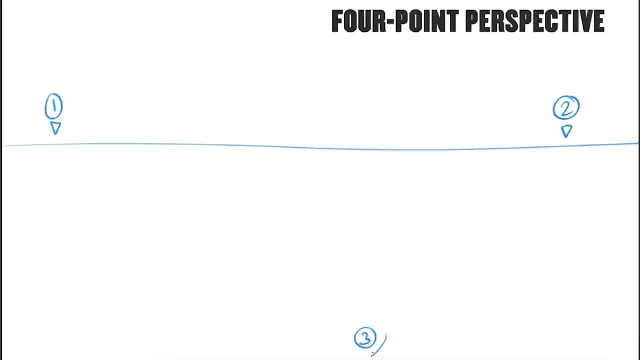 it has four points. Now, like I said before, the third vanishing point either goes above or below the horizon line. So that means that this vanishing point, as we have already a vanishing point below the horizon line, this one actually goes above it. So we know where the vanishing 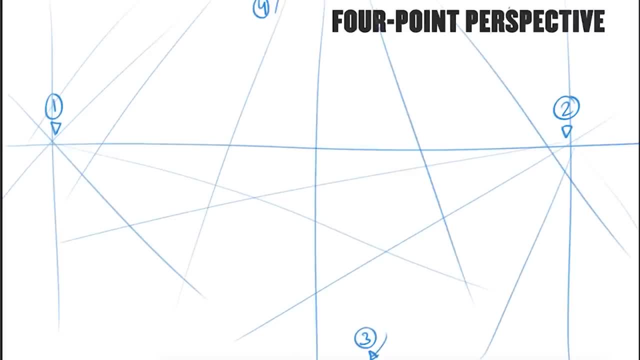 points are. We can draw out radiating lines that create depth And now we have a full scale grid. Now, when we are looking at this grid, you can probably guess this makes for a very difficult drawing, because we have to count for four points whenever we're drawing. Now, when you're drawing a cube in 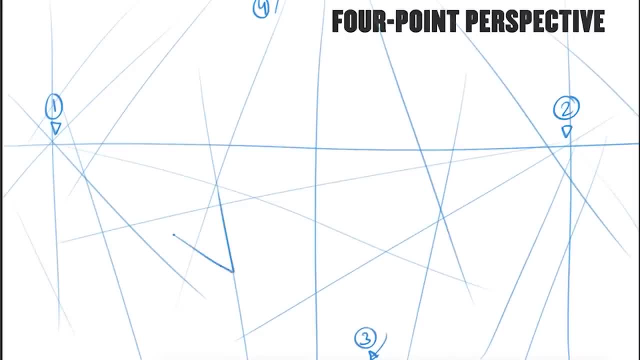 this grid, I always advise you to first put a dot where you're going to aim for with your line. If you don't do this, you have to think about the angle and location of your line, which is almost impossible, So it's always handy with dots before you start drawing a box or anything in this. 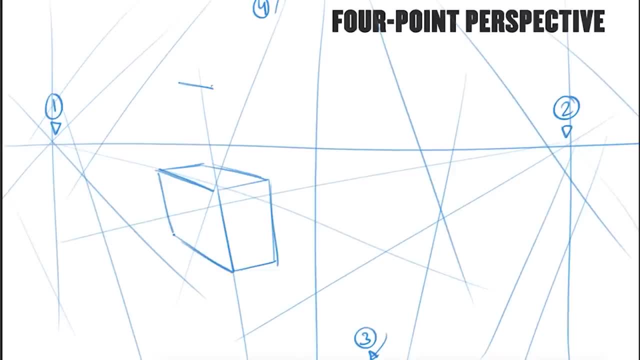 grid. Now what you'll see is that the boxes that go below are going towards the vanishing point below and the boxes on the top are going towards the vanishing point on the top. This also means that we kind of look on boxes which are under the horizon line and we look on two boxes We can see. 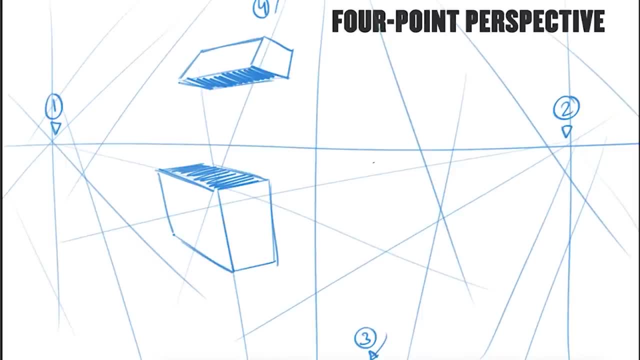 the underside of boxes if they are floating in the air. Now what happens if a box is overlapping with with the horizon line? then all the lines are actually converging to their vanishing points. So that means that both the top and the bottom are converging towards the third. 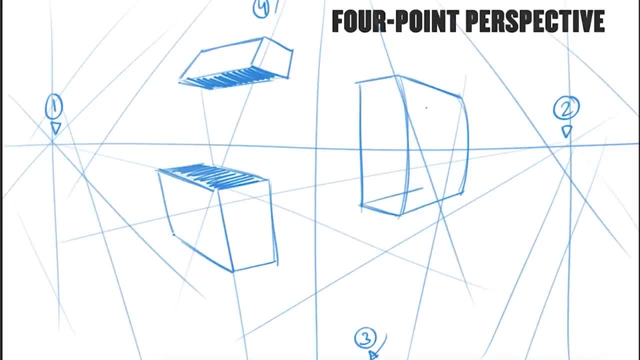 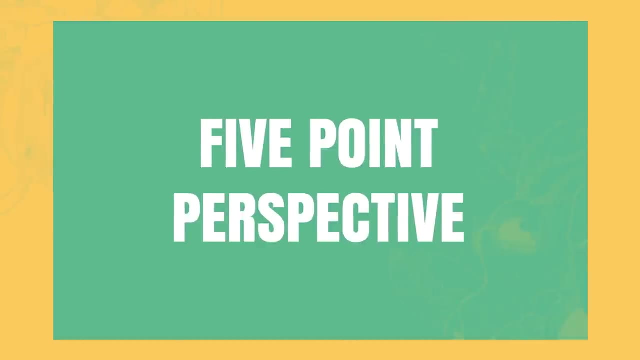 and the fourth vanishing points. So this means that actually the lines are getting a little bit curved And this is already the beginning for getting towards a curve, linear perspective for a five point perspective. Now, a five point perspective is actually quite similar from a four point perspective. 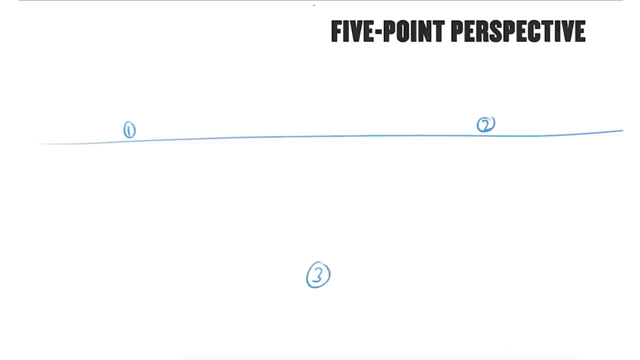 We have the vanishing points one, two, three and four And if we connect the third and fourth vanishing point with each other, we have the four point perspective. but we're just adding a fifth vanishing point in the middle. 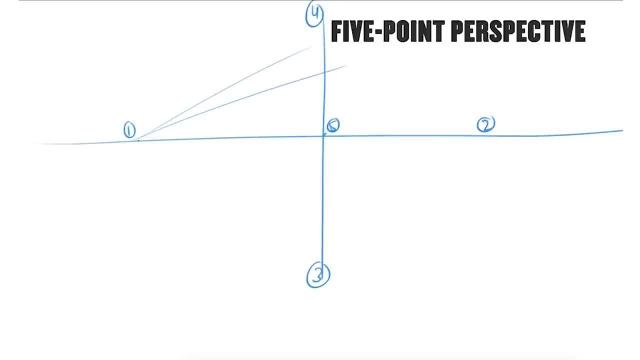 Now, instead of using straight radiating lines from these vanishing points, we're gonna use curve, linear perspective Curved lines, And that means that they start at number one and end at number two, or the other way around, And the same happens for the vertical ones. 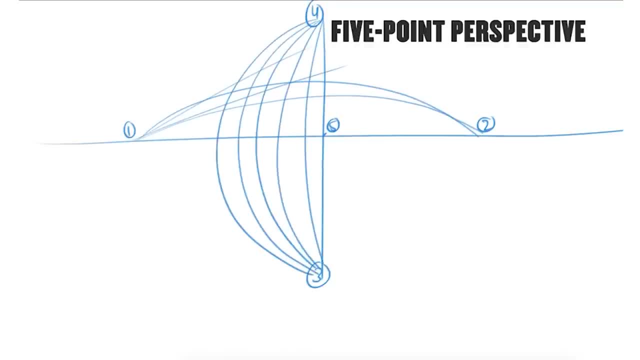 Start at number four, end at number three and the other way around. And the more these lines move away from the fifth vanishing point, the more curved they get. You can actually say that there is a circle around this grid- Only the lines that are from the fifth vanishing points. 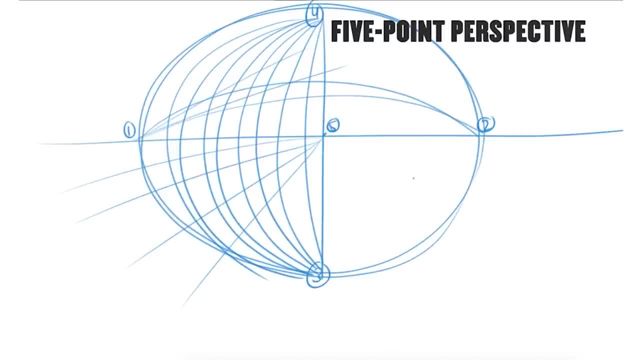 are straight, But actually this is not true, because this is how we view the world. This is how we view the world. You could actually say that we're standing over here and we're looking at the world with a round view. right, This is this. 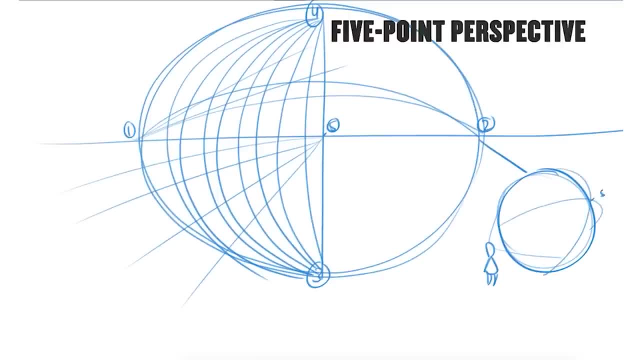 And what we see is this And the fifth vanishing point which is over here. these lines are actually going around us And they also have a point where they meet another vanishing point, which you could say is the sixth vanishing point. 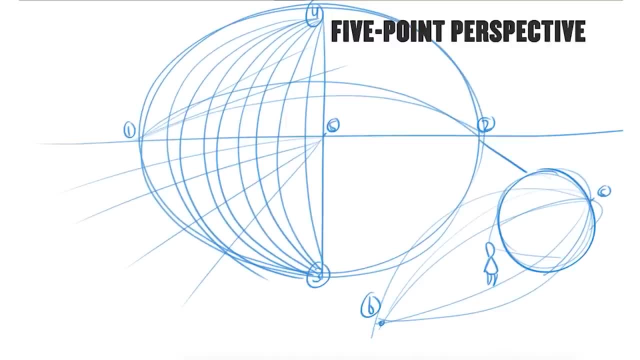 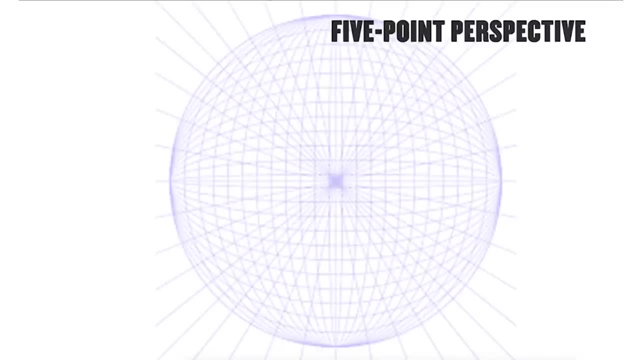 This is the vanishing point. we don't see. You can forget this, because you're not using this in drawing, but you are gonna be using this grid, or at least Kim Young-ji does. Now this looks very complicated, but if we make it a little bit more simple, 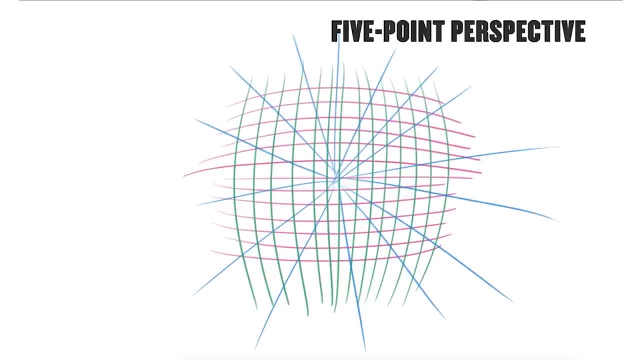 like this and we take away the grid, then you can actually see that this grid is very similar to a one point perspective. The only difference is that these lines- the pink and the green lines- are just curved a little bit. If you train yourself in using a one point perspective, 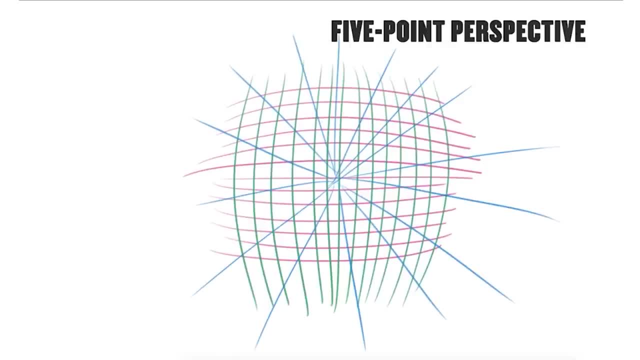 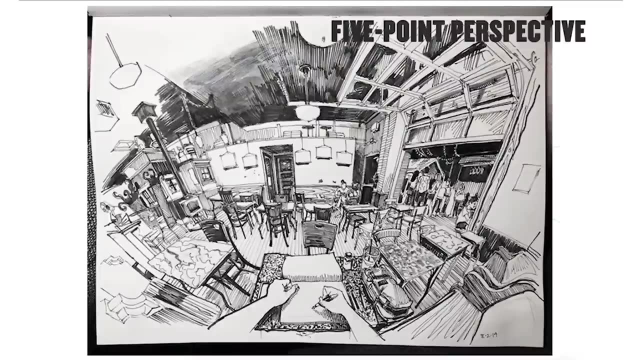 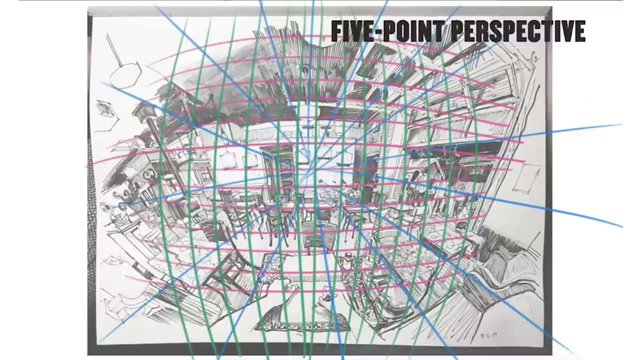 and instead of using straight lines, you use curved lines. you're already using a five point perspective. Now, someone who's very good at this is Paul Heaston, So check out his Instagram because he makes these awesome five point perspective drawings that if we overlap this grid with the drawing, 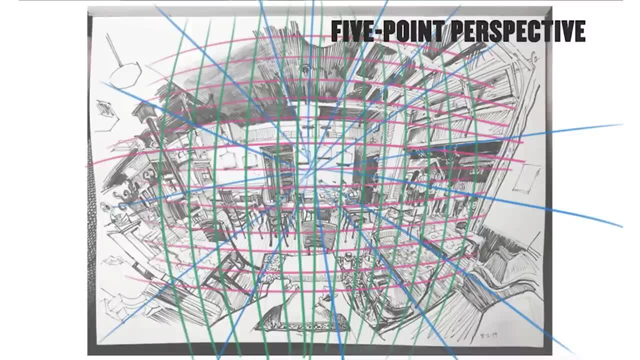 you can actually see that it gives a little bit of guidance to how to look to the world. Another way of how people describe a five point perspective is saying they use a wide angle lens. So let's have a look. Let's have a look on how lenses influence our perspective grid. 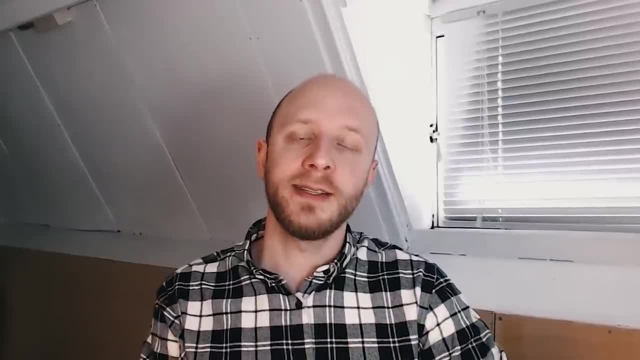 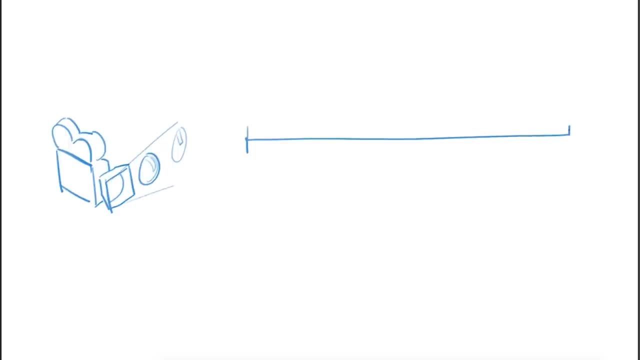 Lenses come in a wide variety, And the reason we're talking about lenses is because lenses have a big influence on our perspective grid. Now, you could say that lenses could be placed on a scale going from a narrow angled lens towards a wide angled lens. 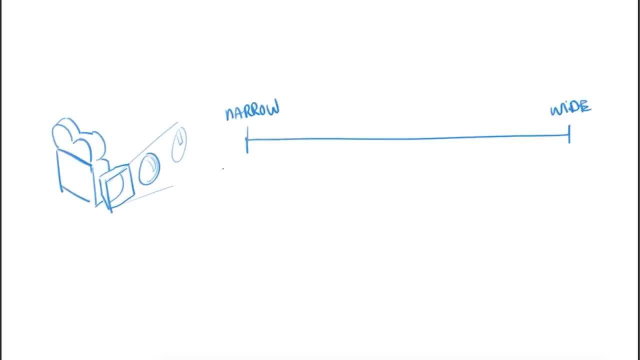 Now, a narrow angled lens is, for example, a 70 millimeter lens, Also known as a telescope lens, And a wide angle lens, or fish eye lens, is around a 15 millimeter lens. Now, now don't ask me about these numbers. 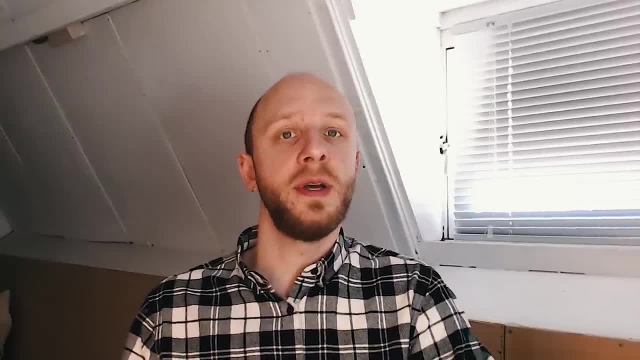 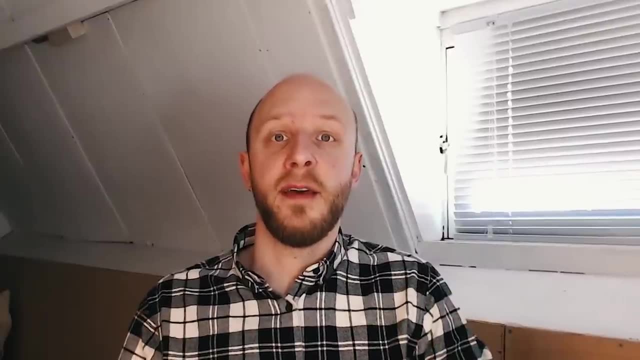 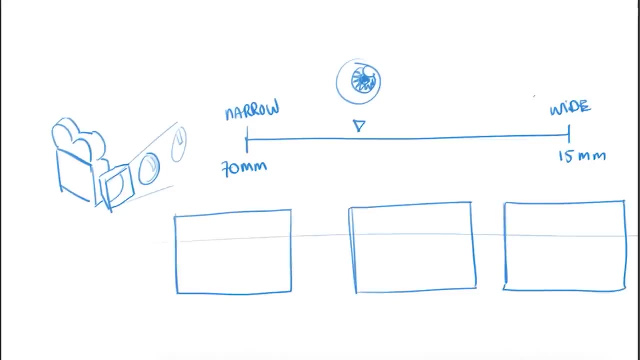 because I don't know where they come up with this, But what I do know is that our eyes have approximately a 55 millimeter lens. Now what does this effect have on our grid? If we draw three frames underneath this scale, you can actually see that when we draw out these grids. 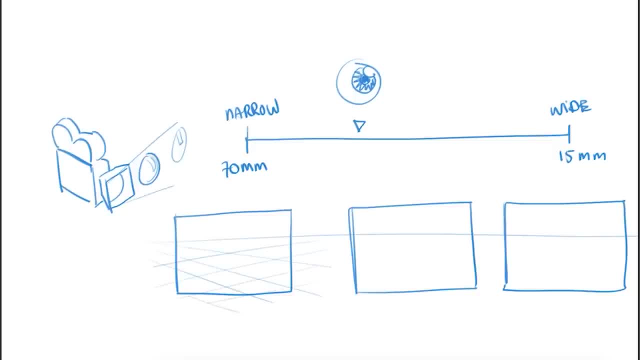 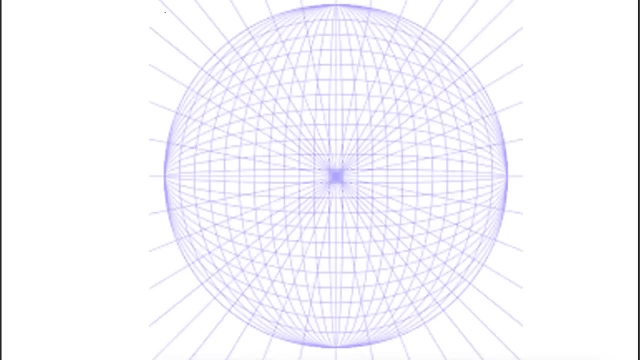 is that the grid for a narrow lens has vanishing points that are very far away from the frame, While when we move more towards a wide angle lens, these vanishing points come into the drawing or into the frame. Another way of explaining this is by looking at the fish eye grid that we used earlier. 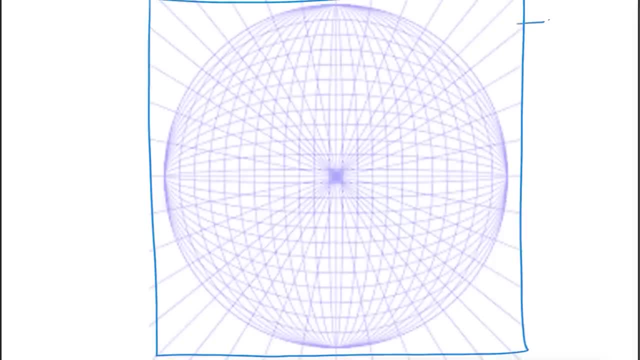 If you're using the whole grid or the wide angle grid in your drawing, then you're using a wide angle lens, But if you're using just a part of this grid, then you're actually using a narrow angled lens Because, as you can see over here as well, 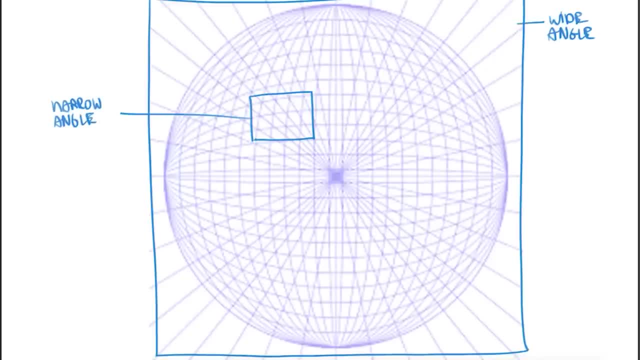 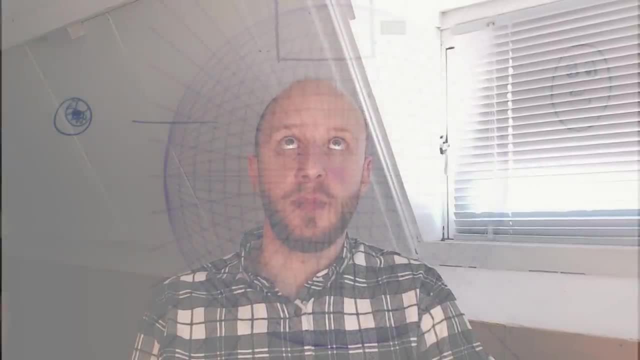 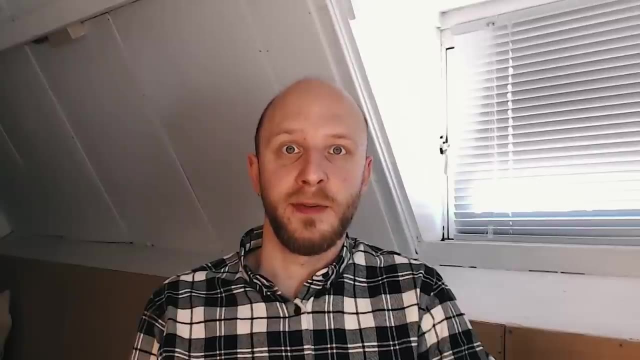 the vanishing points are further away. they're not in the frame. So if we imagine this grid being our head and we look up, the frame goes up, And then when we look down, the frame goes down. And if we look straight, 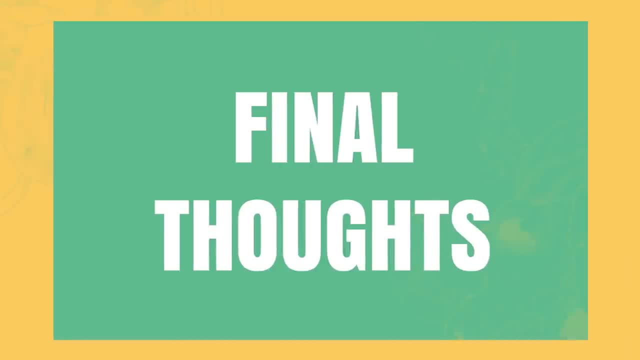 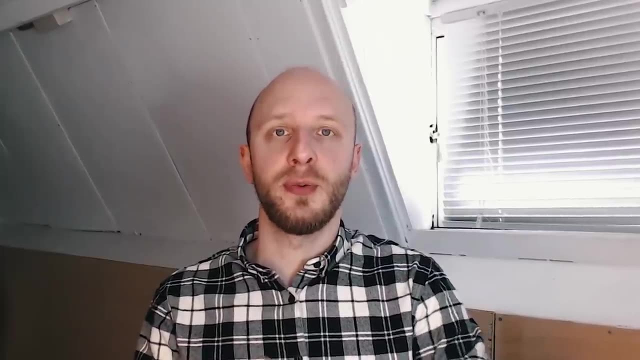 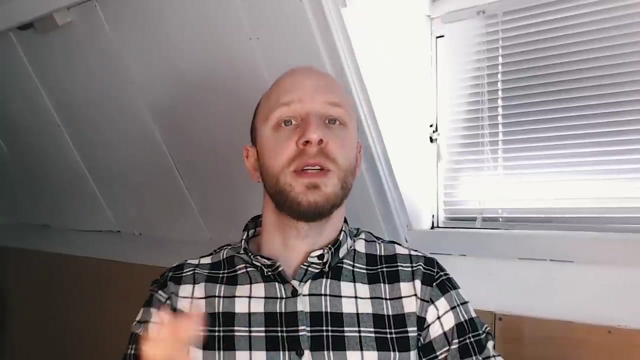 the frame goes straight And I see you guys. The final thought I want to share with you guys is the difference between the horizon and the horizon line. Although they sound very similar, they are actually pretty different, And let me show you this with an example. 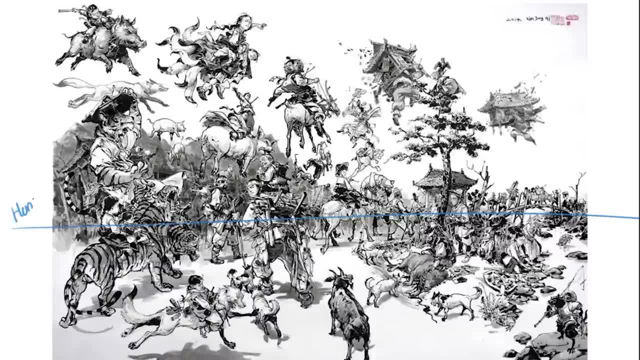 You'll see, here in the middle, we have the horizon right. This is where the sun sets and the moon rises, And all the objects that are standing on the ground are actually following the rules of the horizon, For example, this goat here. 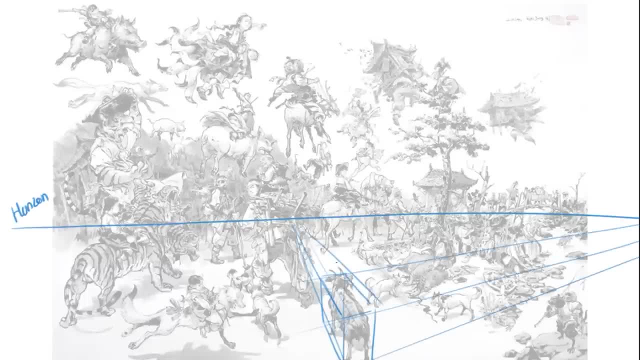 If we draw a box around him, you can actually see that there's a vanishing point here on the horizon And there's a vanishing point somewhere off the page. But all the objects which are above the horizon, which are floating in space,